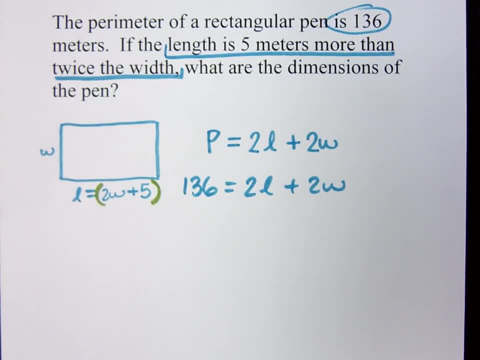 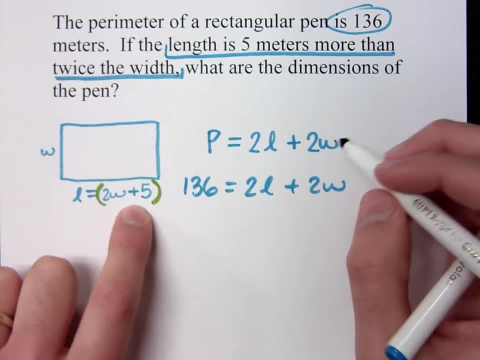 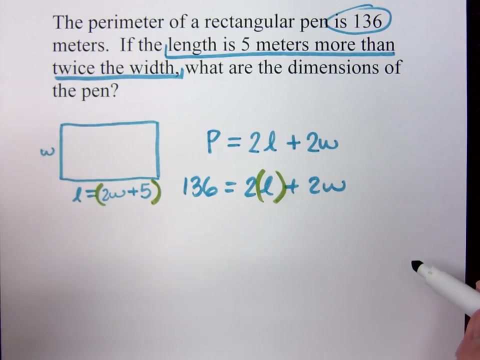 That's what we have right here. The length is 5 more than twice the width. do with this is that in this equation where I have two unknowns, I can take out that L and put in what the length is, just like we had with those other. 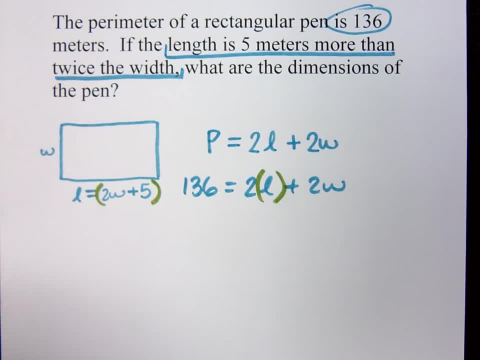 problems with the like with the triangle or the board that's cut into different pieces. we can do that here. so the 136 is equal to 2 times my length, but my length is based on the width. so what is the length equal to? to W plus 5, right? the? 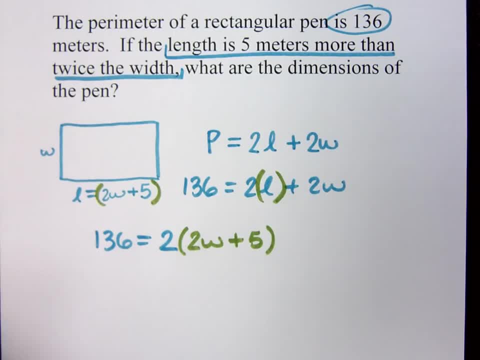 length is not just twice the width, it's twice the width and the 5 meters more than that and plus 2 W. so look what I did. the width is still the width, but my L is what read it. the length is is five meters more than twice the lid. Now notice what I'm not doing here. I did 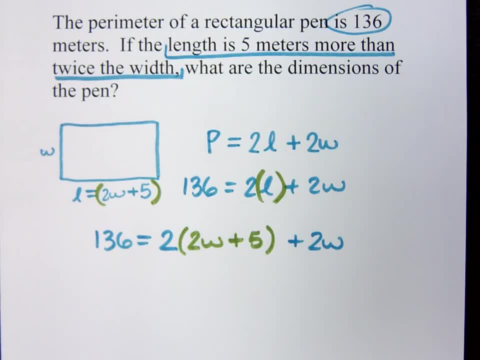 not introduce X at all, did I? When you're using a known formula, you don't need to tell me what L and W are. It's obvious what they are. It's known what they are, what they represent. So now I have 136 equals. what? 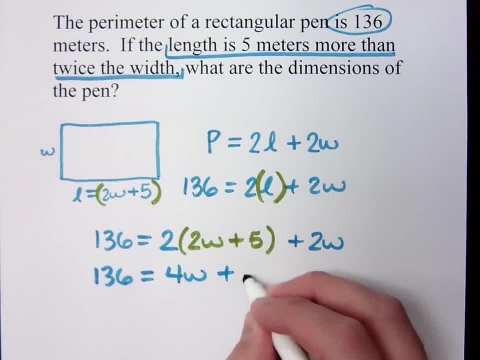 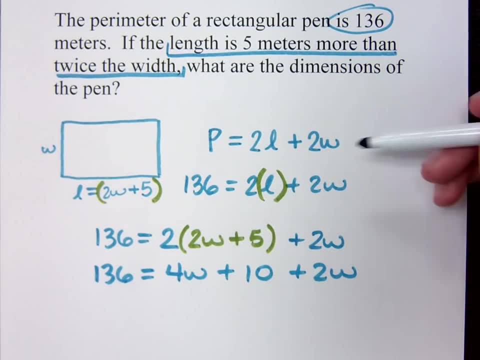 4W plus 10 plus 2W. See, I had three variables at the very beginning, but you knew that P was 136. That left me with two variables, which still was not good enough for what I'm talking about From here. once I replace my length with 2W plus 5, I only have one variable. 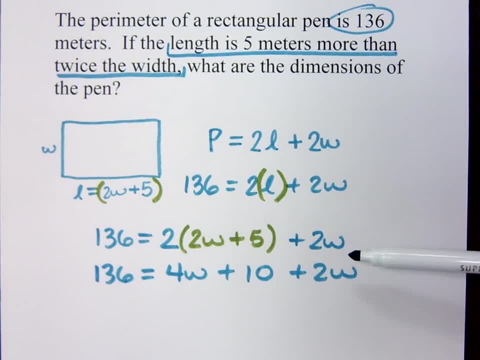 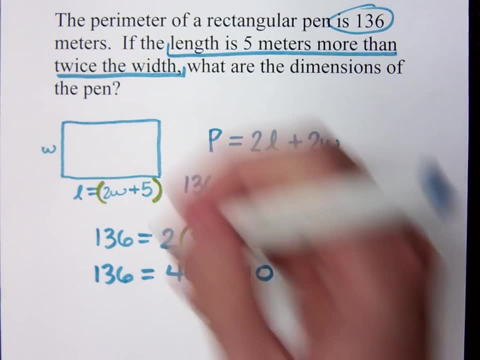 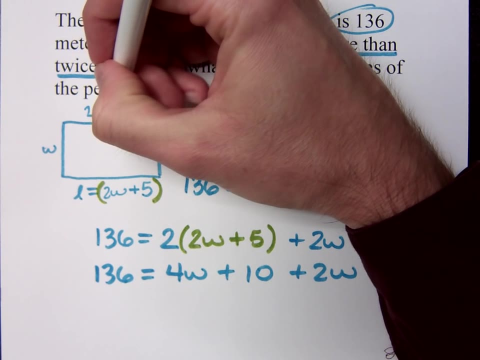 I may have multiple variable terms, But I only have one unknown, which is my width. Now understand what you have with rectangles. This side, over here is W, right, And up here is another length, which is 2W plus 5. Do. 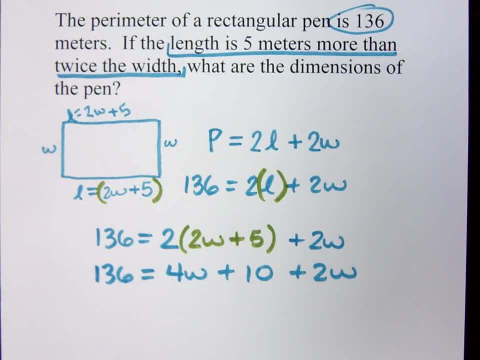 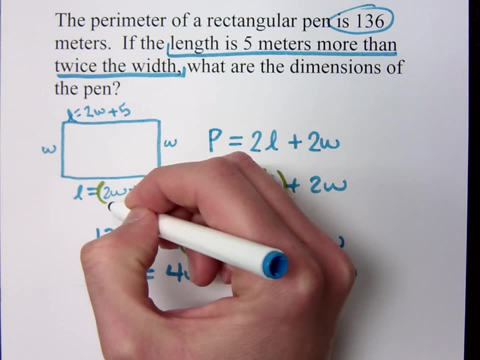 you agree? Perimeter is the distance around a figure, Do you all agree? So W plus 2W plus W plus 2W plus 5.. Okay, W plus 2W is how much? How many W's do we have if we go all the way around here? 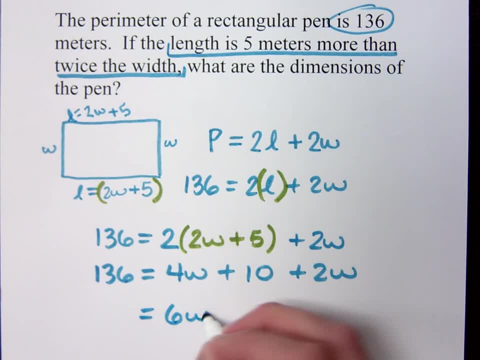 Six, You have 6W, and then you've got plus 5 and plus 5, which is what Ten? Isn't that the same thing that we have in our equation? 6W plus 10?? So if what, I'm. 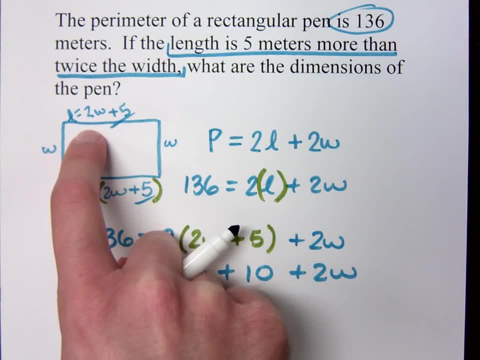 doing here seems confusing to you. you've got your diagram and you understand. the perimeter is adding up all of the sides. okay, Yeah, Can you finish solving this equation for me? 29? And I'm going to cry, right. 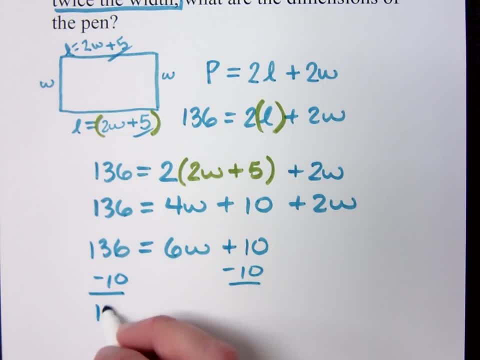 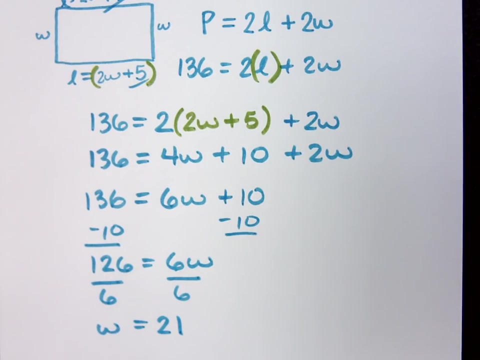 9. Subtract the 10. 126.. 126 equals 6W. Right, you've got to find out that W equals 21.. What does that mean? 1 Bitcoin, 2. 10. 30 wallets. 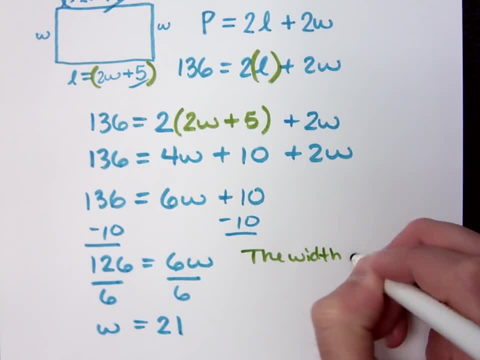 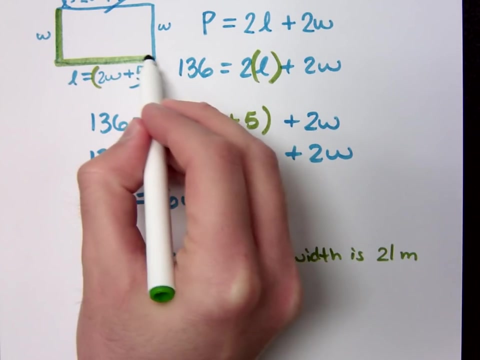 Okay, Yes, width is 21 meters, though right. Say again Times two, When we talk about the dimensions, like if this were representing a room, you would say the dimensions of the room would be this by that, right. So if the room is 21 meters, 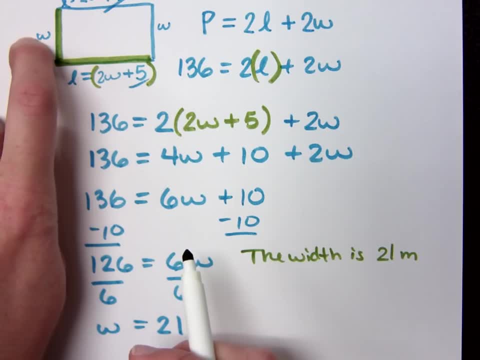 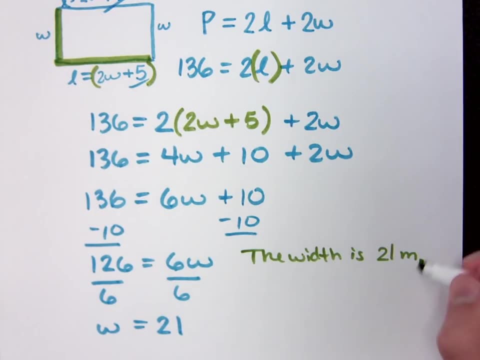 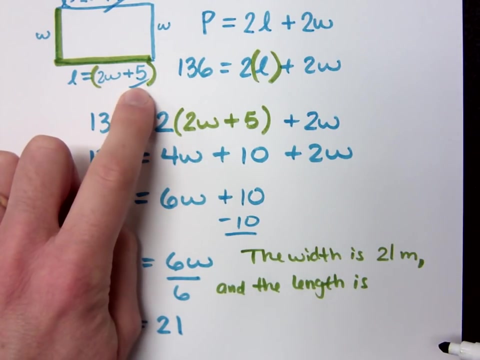 wide. we don't say it's 42 meters wide, it's 21 meters as measured on one side right. Same thing for this rectangular pen: it's 21 meters wide. And what about the length? Exactly right, We said that the length is twice the width plus five. so if the 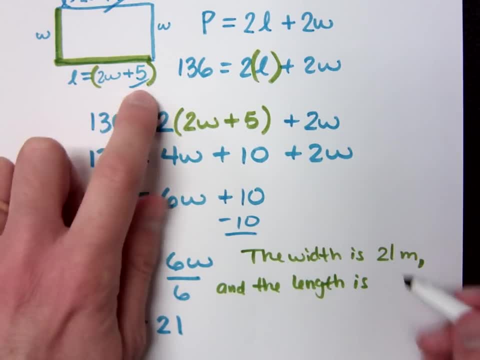 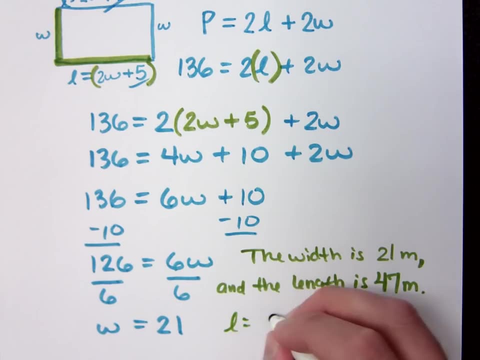 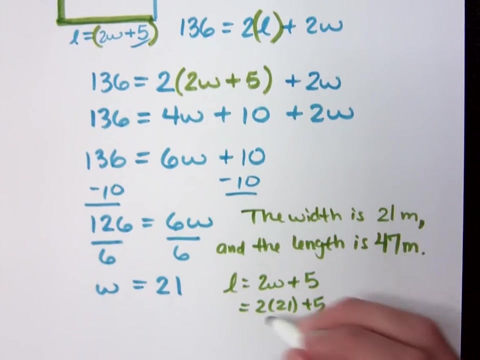 width is 21,. times two plus five should give us 47 meters. right, And in case you kind of didn't see, that that's the length is twice the width plus five. two times 21 plus five, 42 plus five is 47..